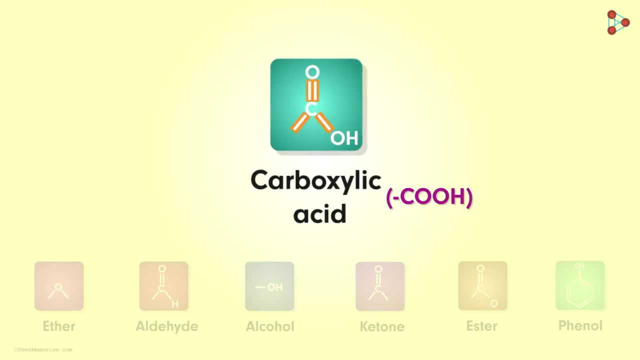 The group contains one carbon atom. Out of the four bonds that it can form, three are already formed, As we can see here. one oxygen atom is attached to the carbon atom with a double bond, while another single bond is with the hydroxyl group. 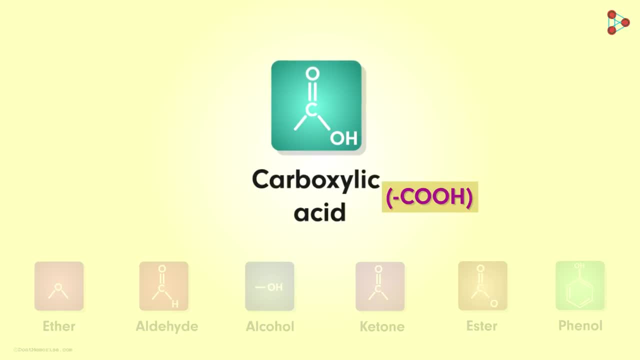 This is how we get COOH and COOH. See you in the next video. Now, from here. where will this group be attached to the hydrocarbon chain? Yes, from the carbon atom. And why is that? We know that the valency of carbon is 4.. 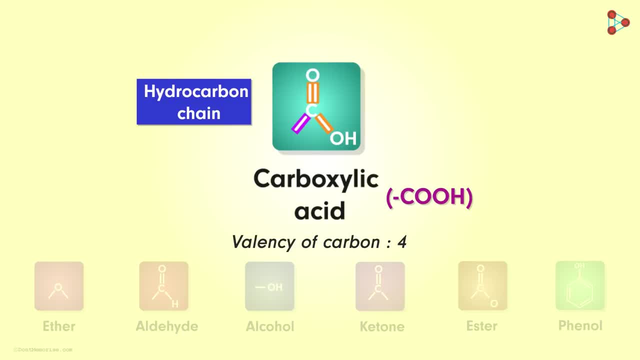 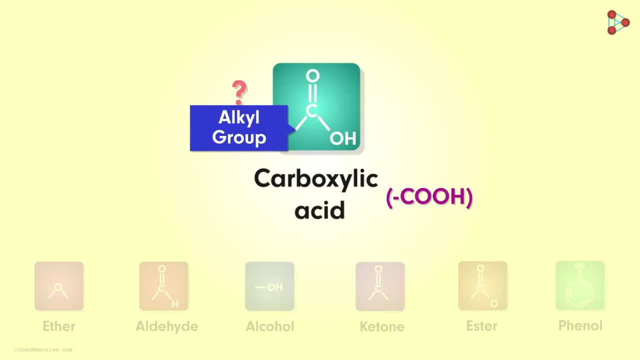 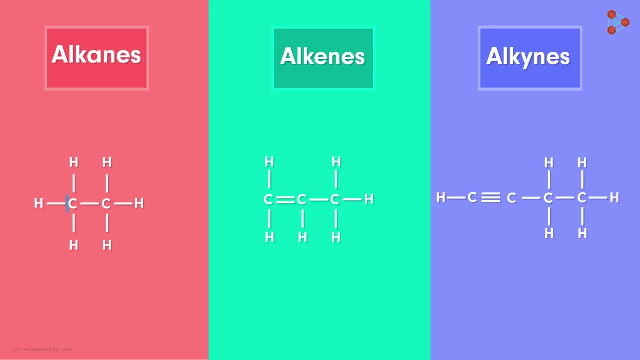 It can be attached to the hydrocarbon chain. It can be attached to the hydrocarbon chain. It can be attached to the hydrocarbon chain. Wait, What do we mean by an alkyl group? We have seen what alkanes, alkenes and alkynes are. 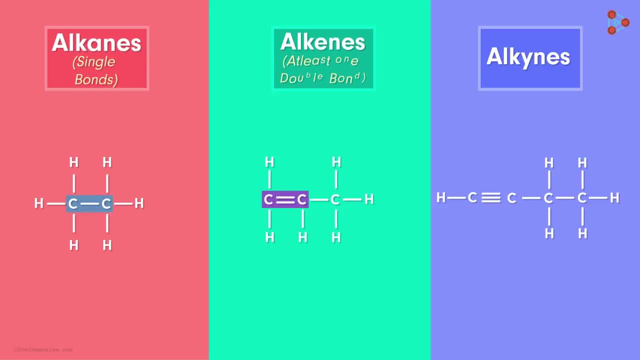 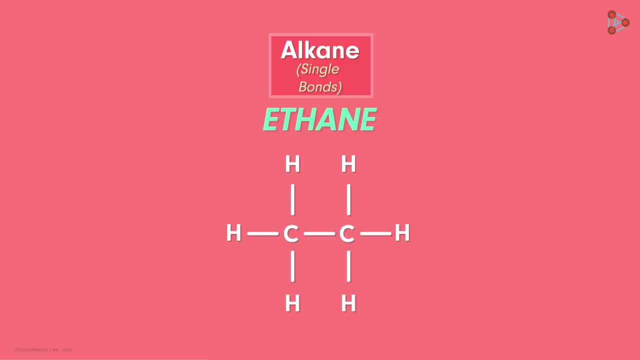 Single bonds, alkanes, At least one double bond alkenes And at least one triple bond, alkynes. So what is an alkyl group then? Let's take an example of ethane to understand this. We can see that each carbon atom here has its valencies completely fulfilled. 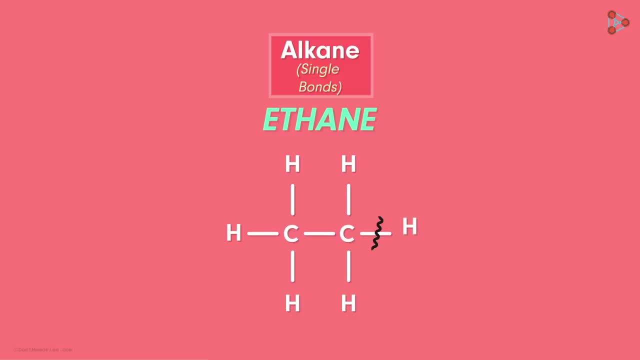 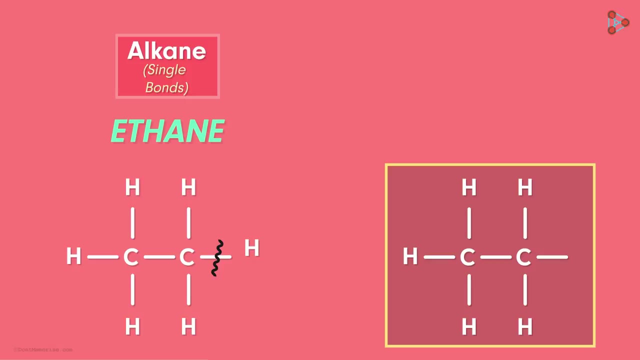 4 and 4.. However, if we remove even one hydrogen atom, then the group becomes capable of forming bonds with other compounds, Like in this case, it can bond with a functional group. from this point, This thing that you see here is an alkyl group. 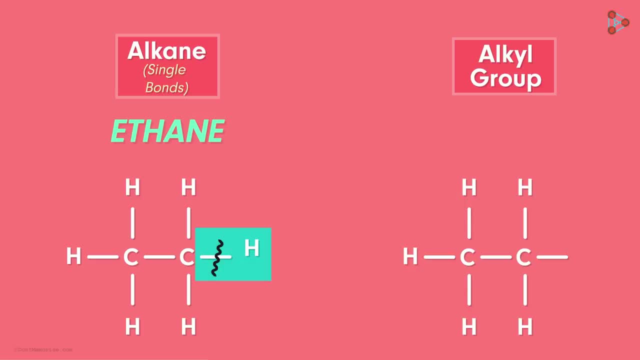 It is just derived from an alkane by removing one of its hydrogen atoms. That's all Here. it is derived from ethane, Hence it is called an ethyl group. Similarly, if we remove one hydrogen atom, then it is called an ethyl group. 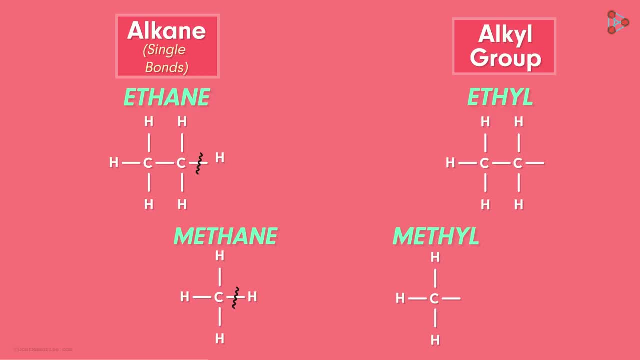 If we remove one hydrogen atom from methane, it will be called as methyl group. Alkyl groups are usually represented with the letter R written in upper case. This was a general overview of what alkyl groups are, But the main topic of this video was functional groups.